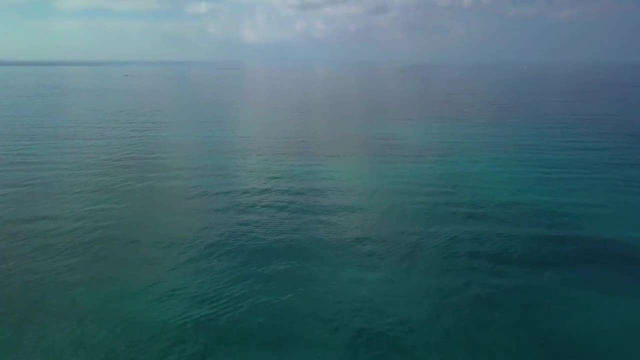 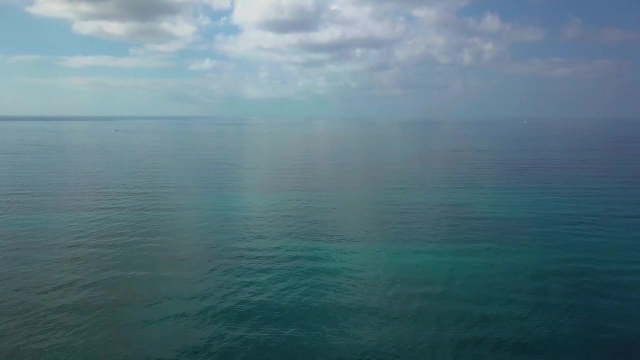 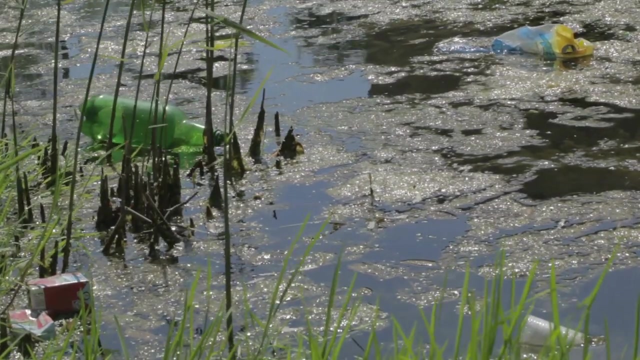 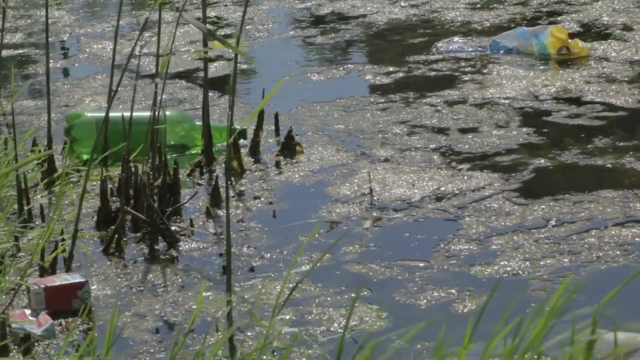 Water pollution has reached frightening levels in recent years, despite the considerable efforts to treat and clean up wastewater. In fact, humans add 1.2 trillion gallons of untreated wastewater into water supply each year. In addition, 14 billion pounds of plastics are dumped into the ocean each year. If we continue polluting our planet with the same, 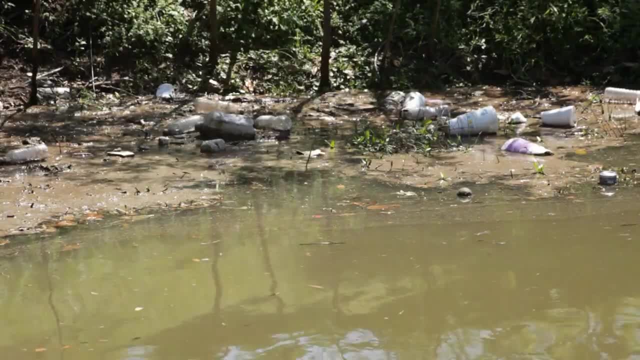 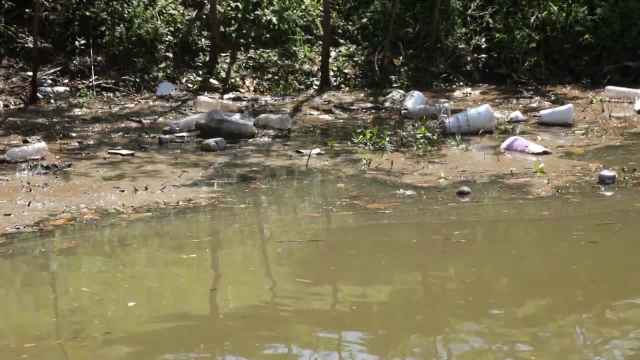 rhythm. 47% of people on Earth will struggle to find drinking water by 2050.. Water pollution effects on human health and environment present serious threats on the future of humanity and our planet. In this article, we will detail the principal effects of water pollution on. 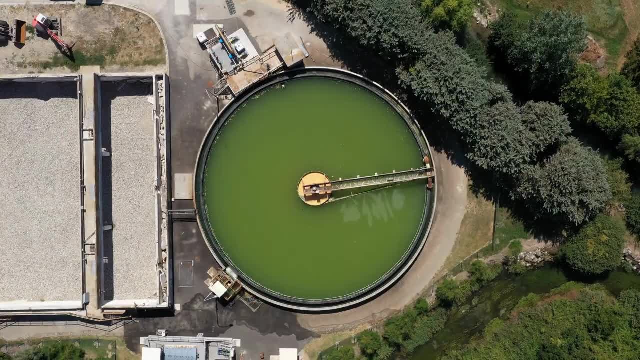 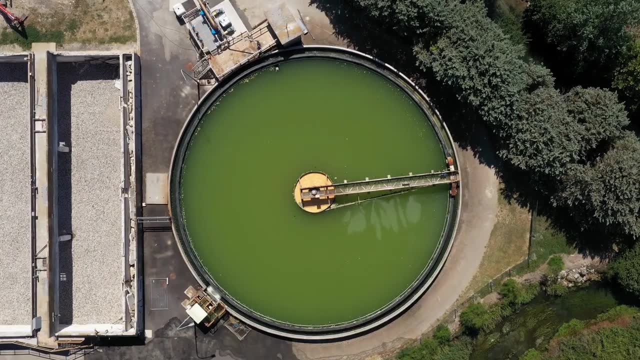 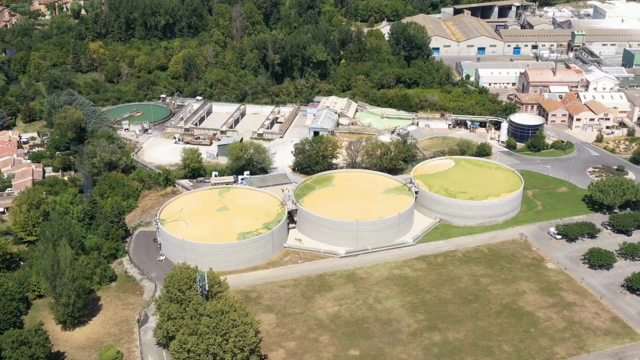 the environment, and we will present some examples of environmental disasters caused by water pollution incidents. There are a variety of water pollution effects on the environment. However, these effects can be summarized in the following elements: The algal bloom caused by water, contamination with nutrients, The effects of chemicals and 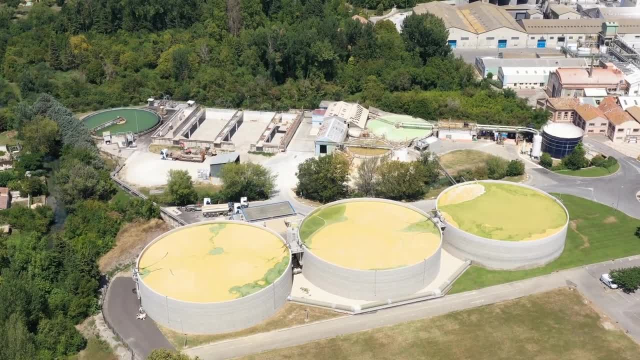 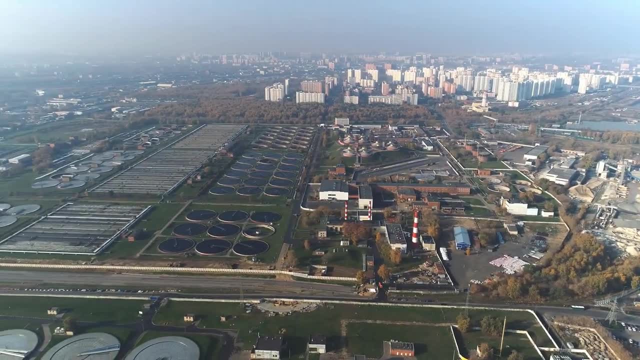 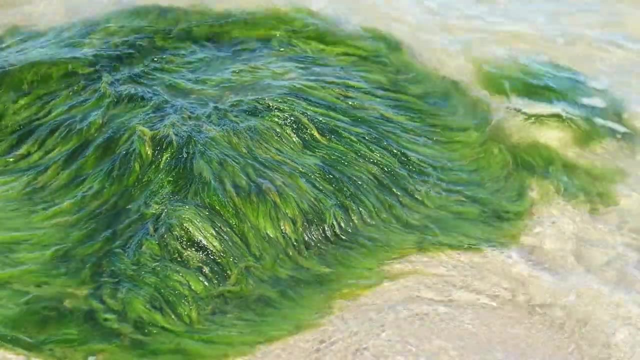 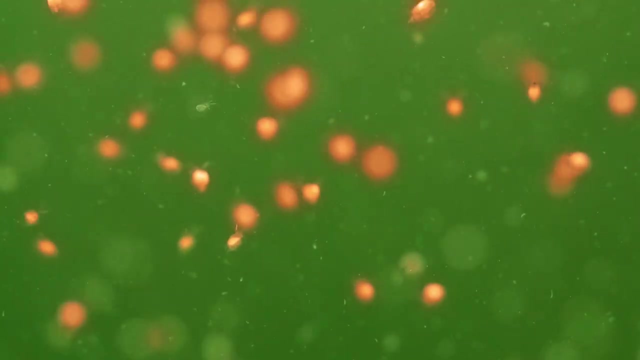 heavy metals on the aquatic life. The threat of aquatic ecosystems by marine debris such as plastic. The effect of ocean acidification on many marine organisms. The algal bloom. The contamination of water in lakes or marine environments by nutrients used, for example, in the agricultural fertilization induces an excessive growth of plant and algae. 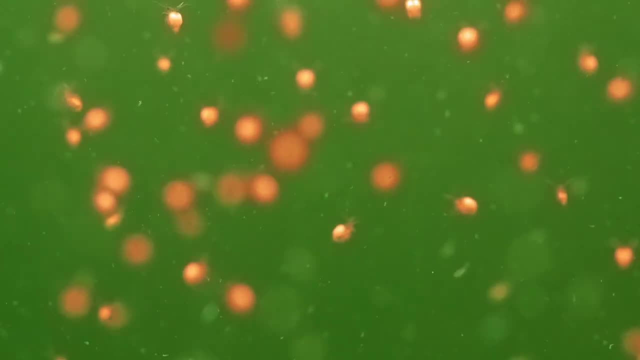 This growth reduces oxygen levels in the water. This lack of oxygen, known as eutrophication, suffocates plants and animals and can create dead zones where waters are essentially devoid of life. In certain cases, this excessive algal growth can also produce neurotoxins that 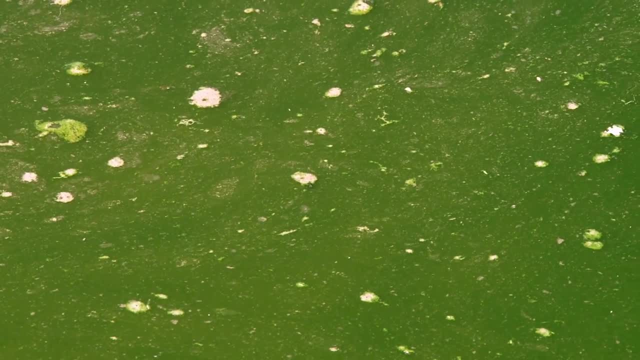 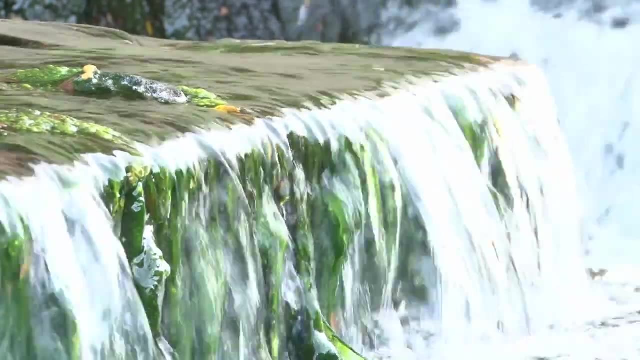 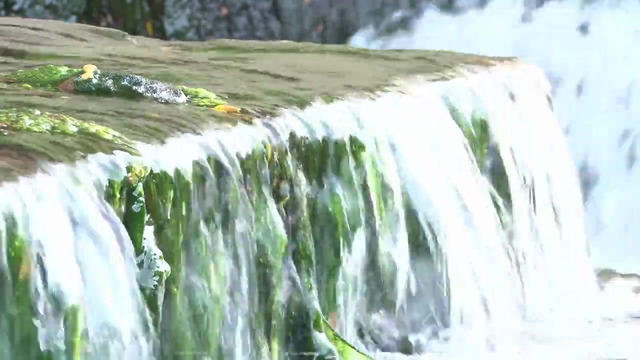 affect aquatic wildlife. Recently, many algal blooms occurred in some regions in the United States. The toxic algae bloom in California's Klamath River in 2017.. The algae bloom on Lake Toledo, Ohio in 2011.. At its peak, the bloom covered 1,930 square miles. 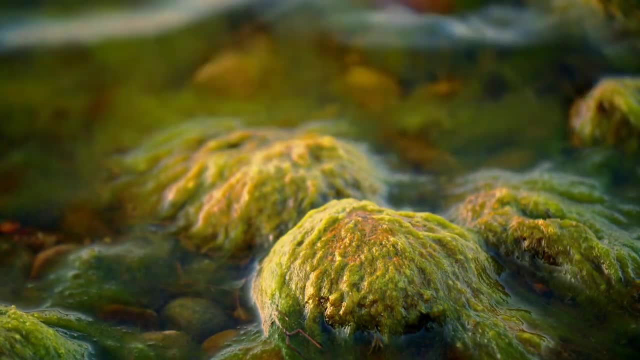 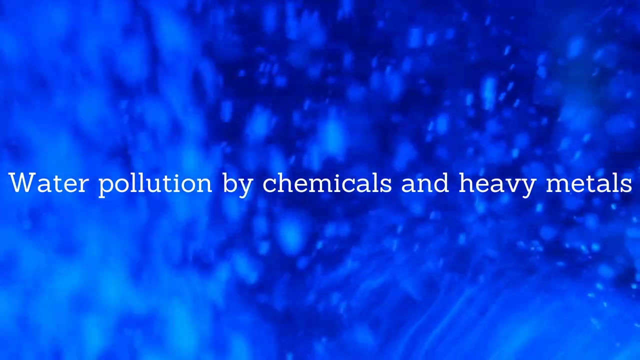 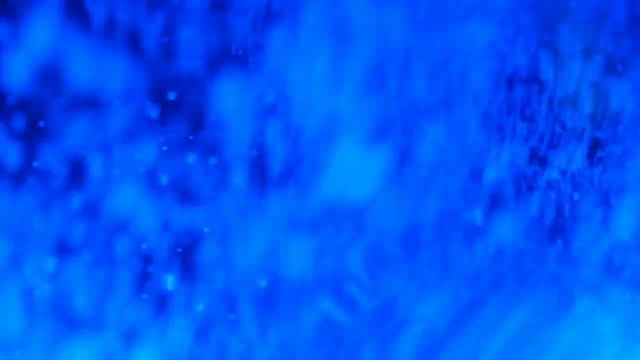 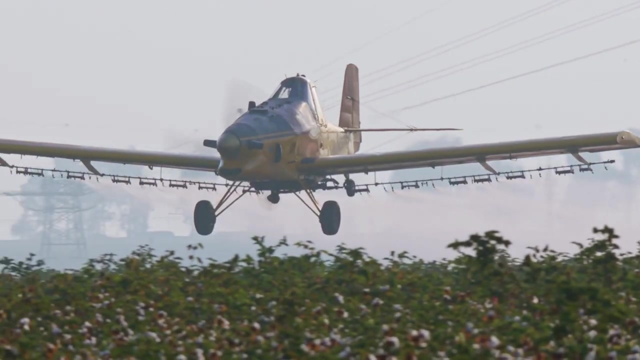 of the nearly 10,000 square mile lake Water pollution by chemicals and heavy metals. The contamination of water ecosystems by chemicals and heavy metals has very harmful effects on the aquatic life. In fact, these contaminants are known to be implicated in the evolution of an organism's life span and its ability to reproduce. In addition, these toxic 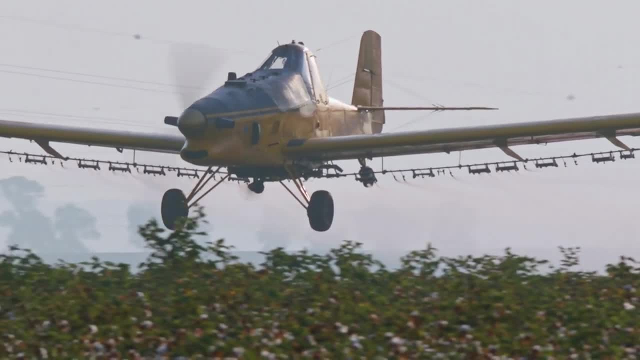 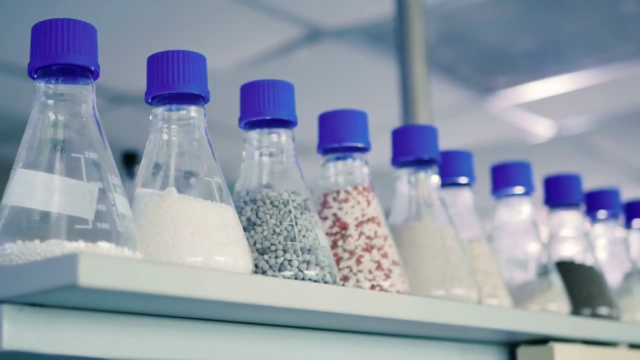 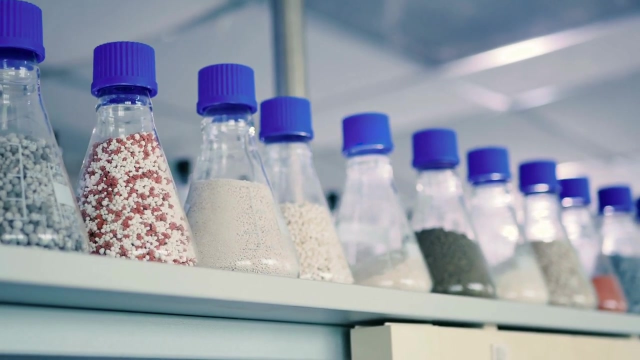 elements make their way up the food chain as predator eats prey. That's why it was reported that tuna and other big fish accumulate high quantity of toxins such as mercury. There are many examples of water contamination by different types of chemicals, and scientific publications are studying new cases every day. However, in this article we will mention only 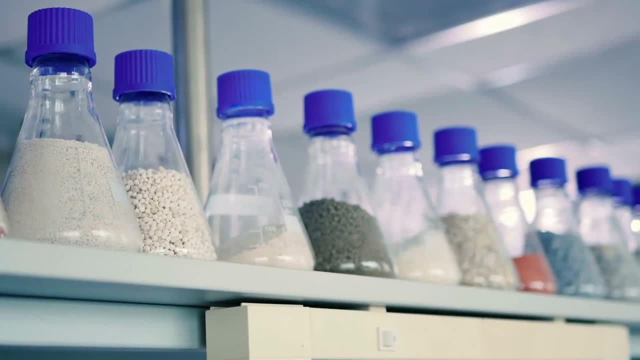 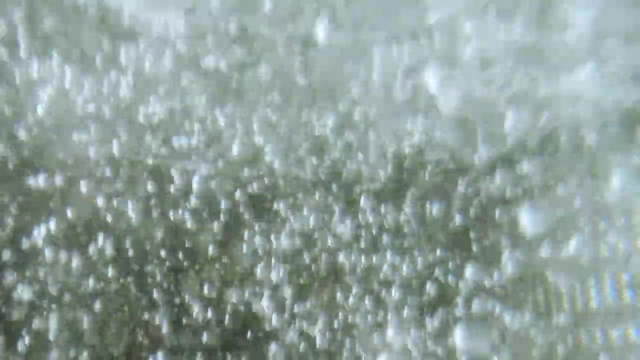 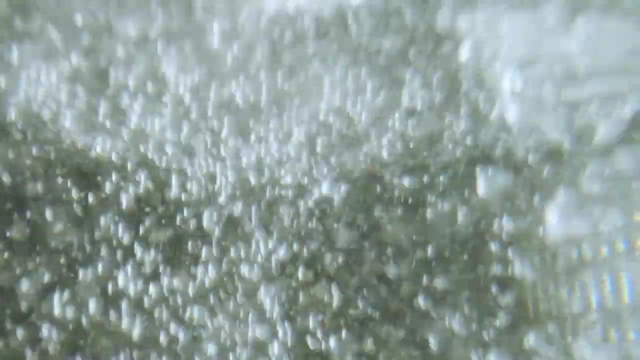 one example with represented a huge threat to our oceans. Seven years ago, the Japanese government was forced to dump roughly 2 million gallons of radioactive water into the Pacific Ocean after the 2011 tsunami hit Water. pollution by oil is also one of the major forms of pollution that is threatening our water resources. In fact, 1.3. 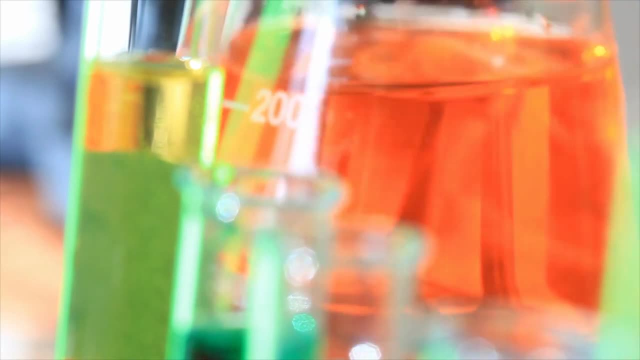 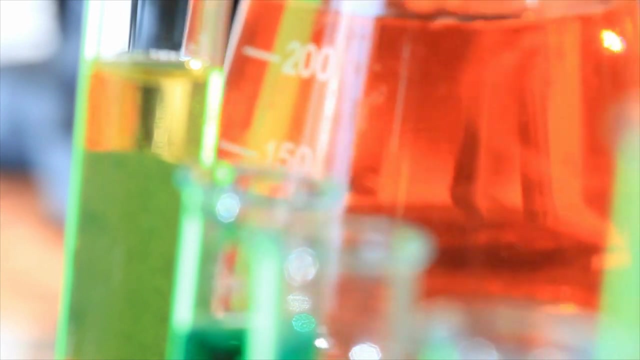 million gallons of oil is spilled into the ocean every year. In addition, for every 1 million tons of oil that are shipped, 1 ton is spilled into the waterways. The world has been wracked by major oil spill disasters many times. The world has been wracked by major oil spill disasters many times. 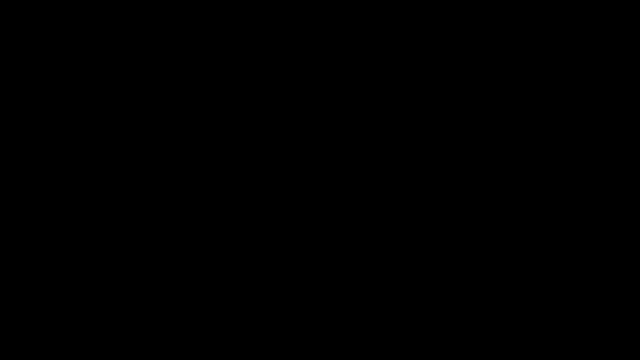 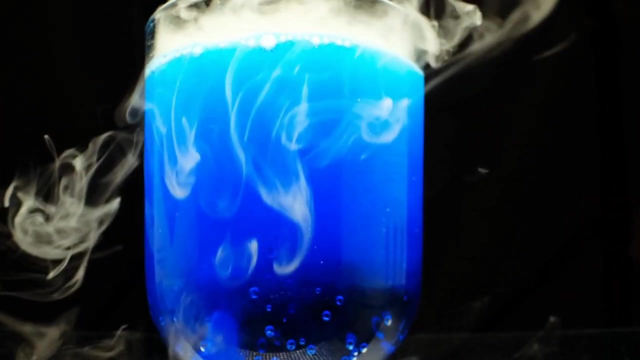 The world has been wracked by major oil spill disasters many times. Here are three of the largest and worst oil spills in world history: The Deepwater Horizon oil spill, also known as Gulf of Mexico oil spill and BP oil spill, and it's considered to be the largest oil spill in the 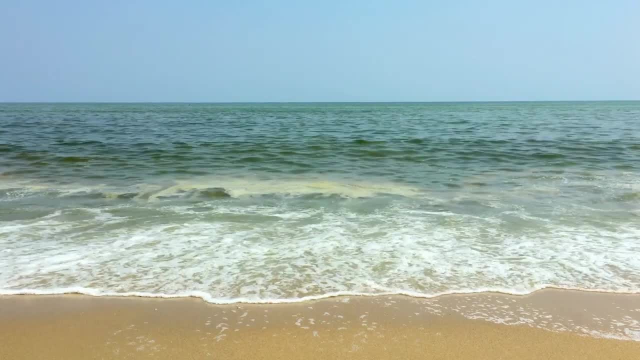 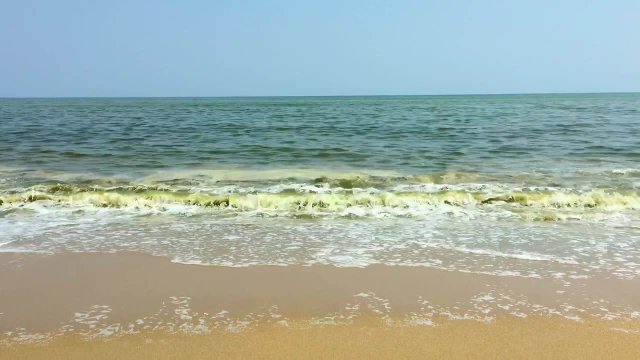 petroleum industry's history. The oil spill continued for over three months. An estimated 53,000 barrels were flowing into the Gulf of Mexico every day. Extensive damage of the marine environment was caused by this disaster. According to the Center for Biological Diversity, the oil 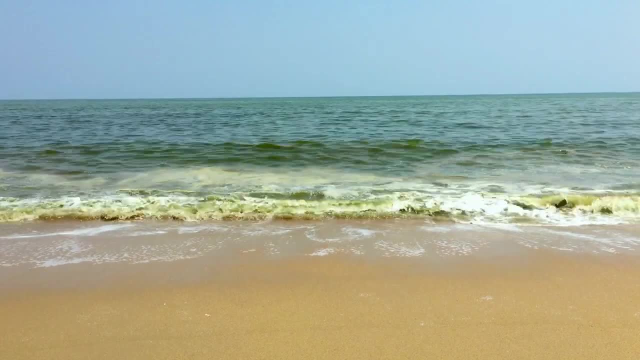 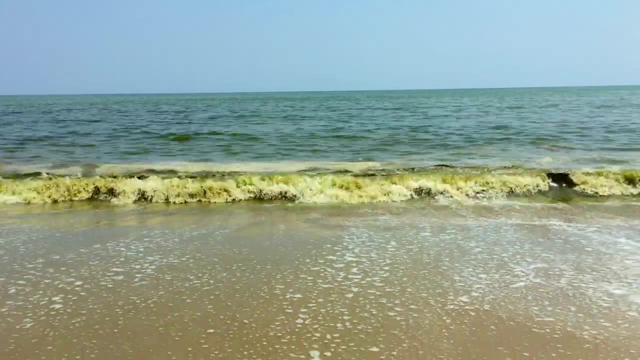 spill killed over 82,000 birds, 25,900 marine mammals, 6,000 sea turtles and tens of thousands of fish, among others. The Bay of Campeche oil spill in June 1979, the Bay of Campeche of the. 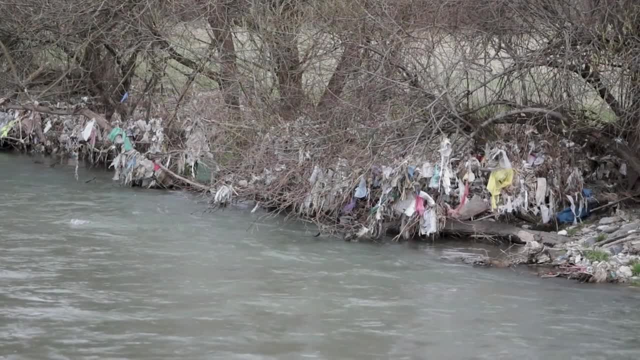 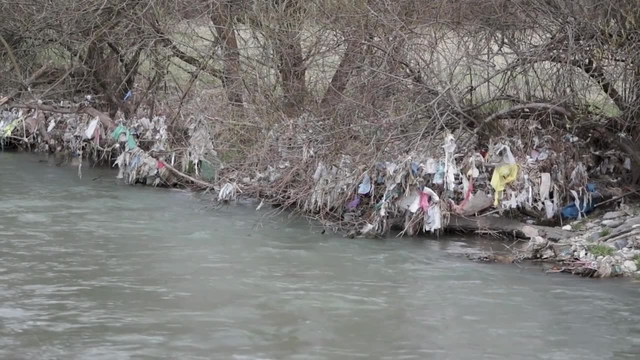 Gulf of Mexico saw the spill of around 140 million gallons oil, almost 10,000 to 30,000 barrels. The oil was discharged into the sea during a ten-months period of time. Exxon Valdez oil spill. it's the second largest oil spill in US history. The oil spill is the second biggest oil spill in the United. 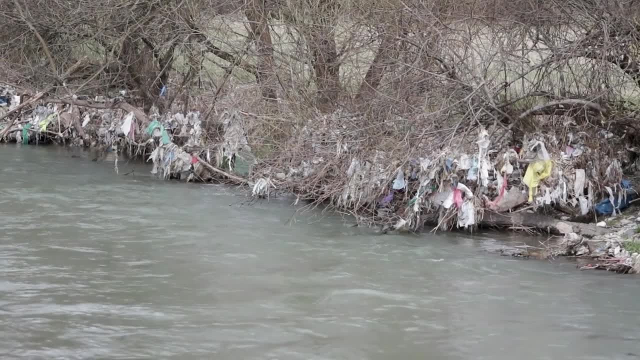 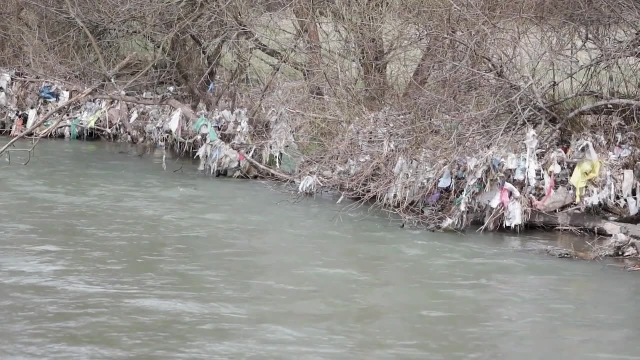 waters in terms of the volume of oil discharged, Due to the accident, which occurred in 1989, 10.9 million gallons of oil were spilled into Alaskan coastline. As a result, the ecosystem in the area was affected badly, as it immediately killed over